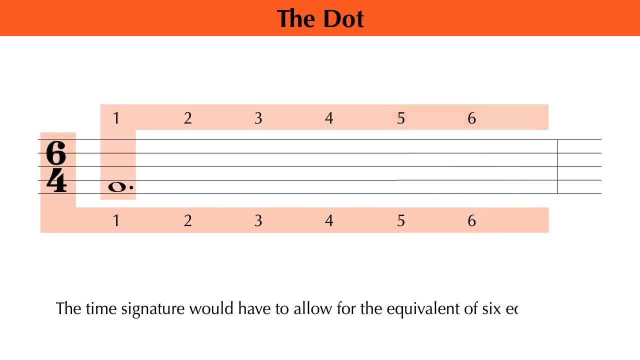 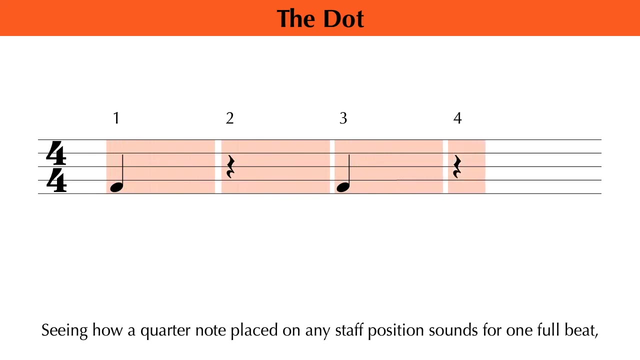 The time signature would have to allow for the equivalent of six equal beats in each measure in order to hold a dotted whole note. Seeing how a quarter note placed on any staff position sounds for one full beat. when a dot is placed next to a quarter note, its duration extends from one beat to one and a half beats. 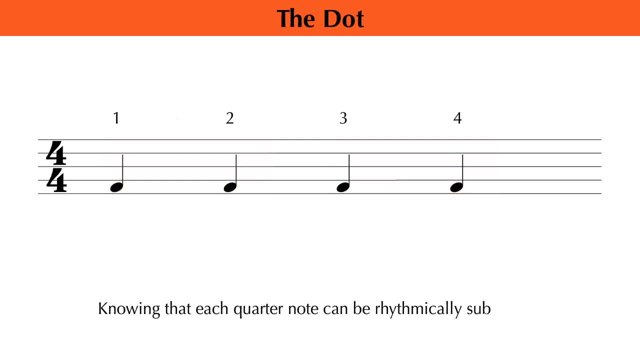 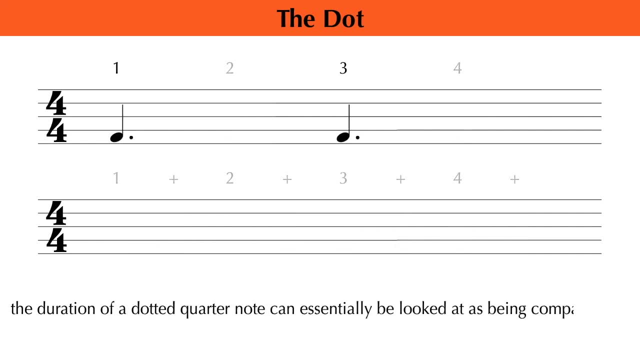 knowing that each quarter note can be rhythmically subdivided into two equal eighth notes, the duration of a dotted quarter note can essentially be looked at as being comparatively the same as the combination of one quarter note and one eighth note. Therefore, when a dotted quarter note is placed on a downbeat, it will pass through the next downbeat and extend until the following upbeat. 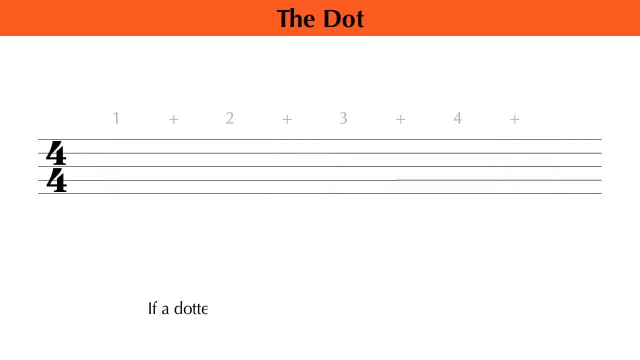 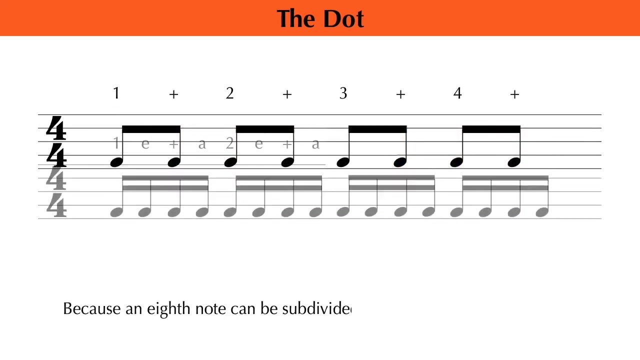 On the other hand, if a dotted quarter note was placed on an upbeat, it would then extend through the following downbeat and upbeat. The next note or rest will be played on the following downbeat. Here is how it sounds, Because an eighth note can be subdivided into two equal sixteenth notes. 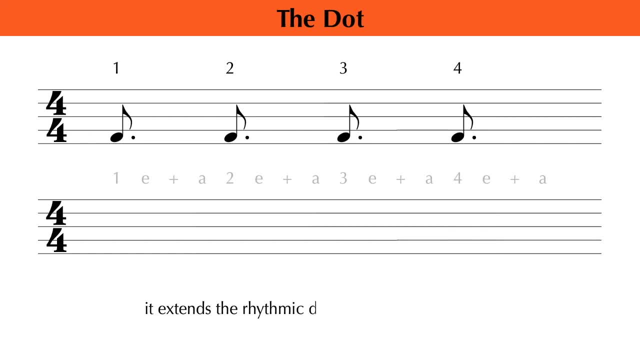 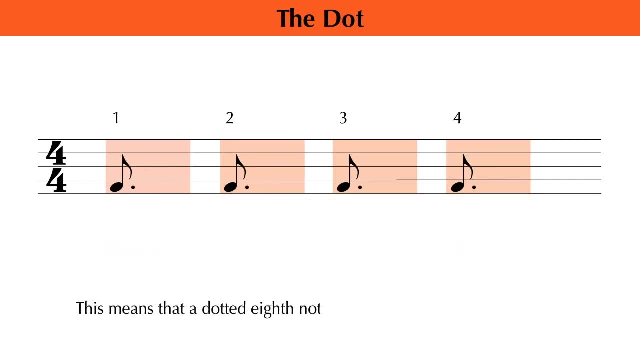 when a dot is placed next to an eighth note, it extends the rhythmic duration of that note to the equivalent of three equal sixteenth notes. This means that a dotted eighth note played directly on the downbeat will be counted by saying one e end. 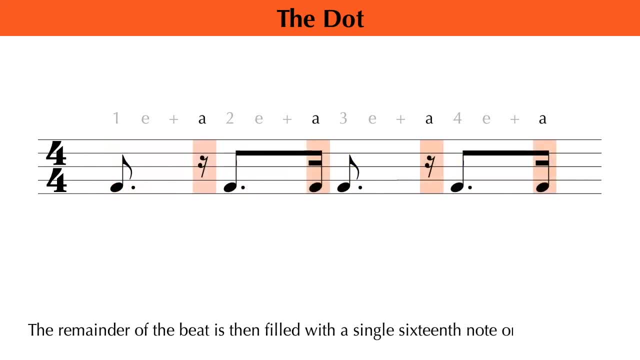 The remainder of the beat is then filled with a single sixteenth note or sixteenth rest. In the following example we can see that beats one and three have been subdivided into four equal sixteenth notes, while beats two and four contain a dotted eighth note. 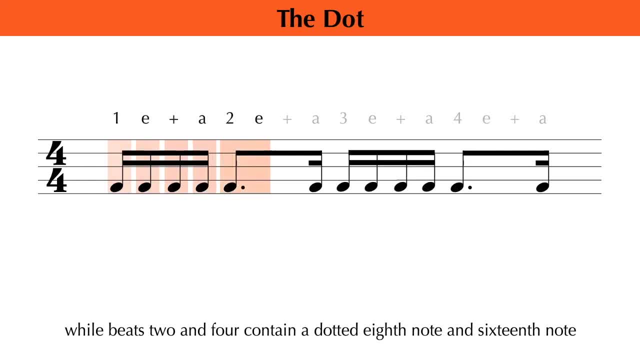 followed by a dotted eighth note and sixteenth note. Now it is also possible to have a dotted eighth note placed on the second sixteenth note. subdivision of the downbeat. In this situation, the dotted eighth note would sustain through the e end ah part of the beat. 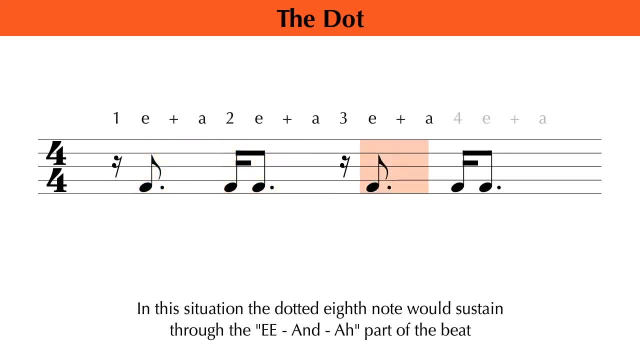 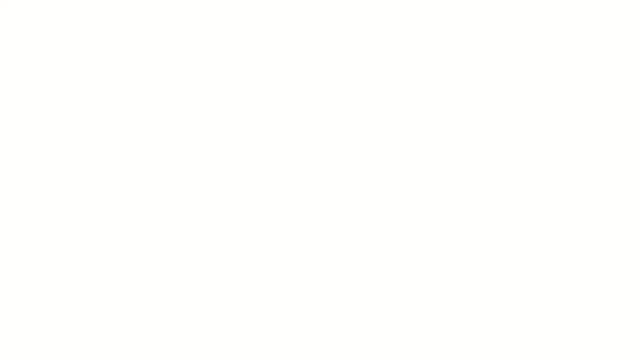 In the next video we are going to talk about the tie. We will see how, like the dot, the tie also extends the rhythmic duration of the note it is connected to.